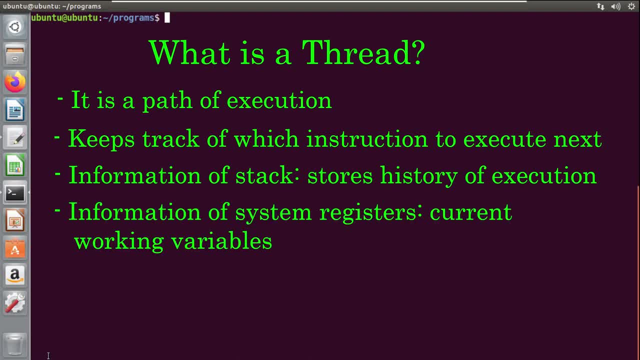 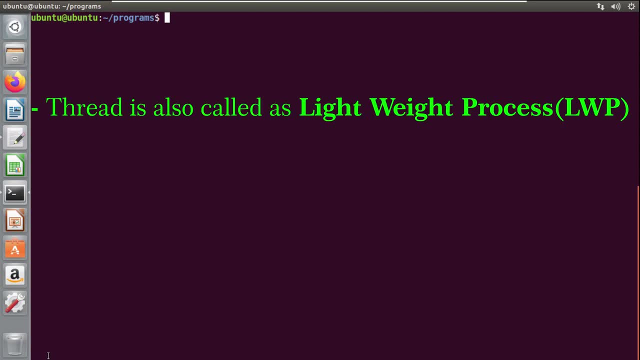 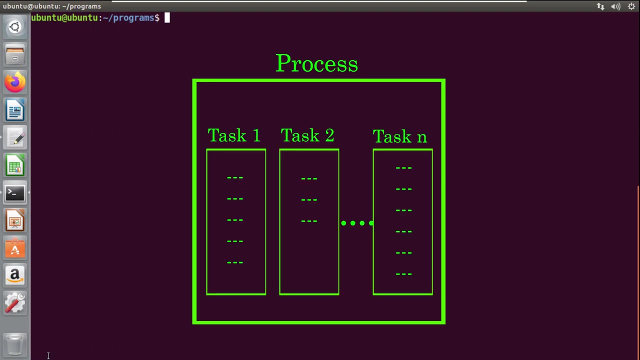 it can contain the information of system registers which have the current working variables. A thread is also called as lightweight process And a process can have multiple threads. Now you may be thinking that we have already learned the concept of process, Now why we need these threads? Basically, a process can have multiple tasks And each of this task is nothing but a thread. These thread improve your application. 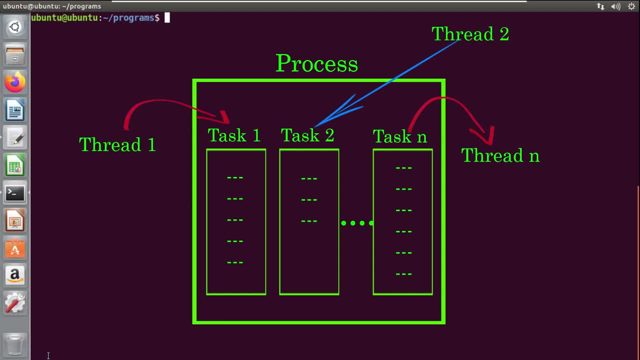 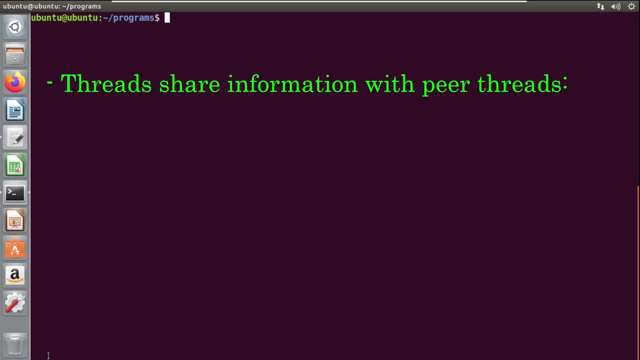 performance through parallelism. This concept is called as multi threading. To give an example, if I say that you might be reading something while watching this video, or you may be having your lunch or dinner, So you are performing different tasks in parallel. So these are nothing but threads. One important point to note here is that the thread shares the information with its peer threads like code segment, data segment and so on. So if one thread makes 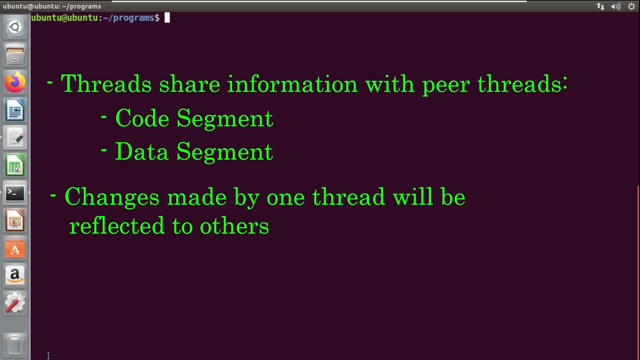 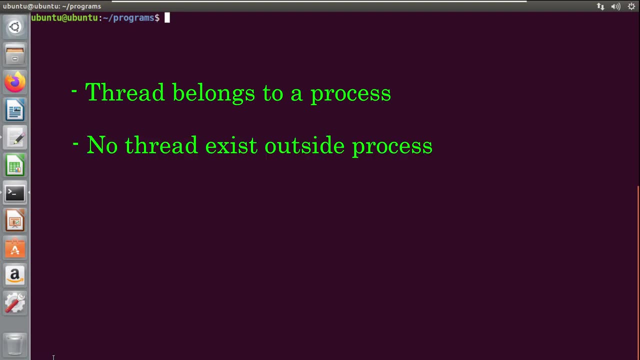 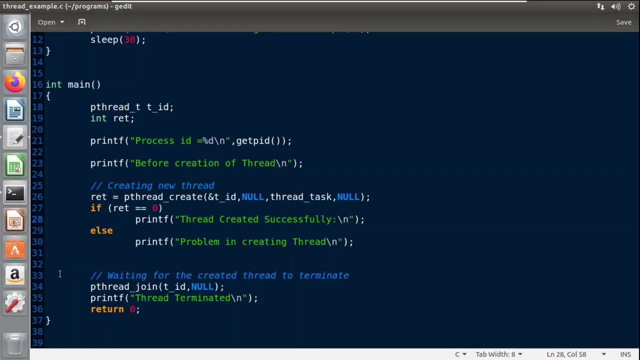 changes in the code segment area, then all the other threads can see that now each thread belongs to a process and a new thread can exist outside of process And so each thread represents a separate flow of control. So there can be a process with a single thread or it can have multiple threads. For example, I have shown three threats here. Now to understand the concept of thread more clearly, I have written a program here in this. 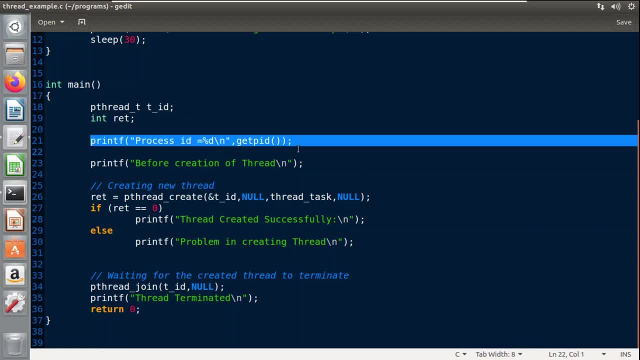 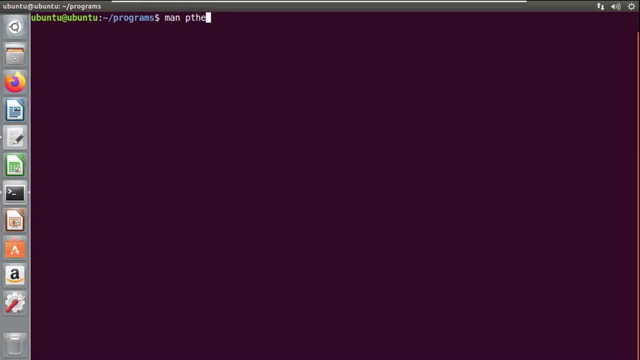 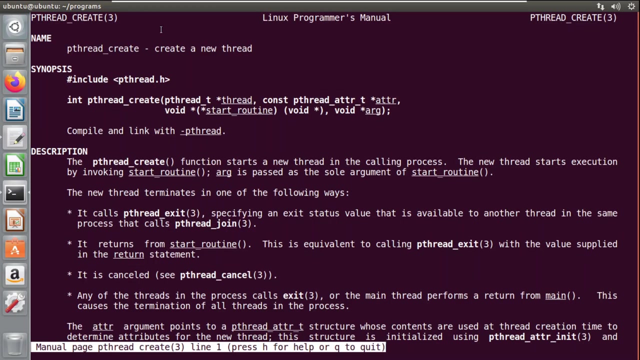 program. first i have printed the process id by using the getpid system call and then i have called the function called as pthread create. now what this function means. we will check the manual page of this function. so man and pthread. pthread underscore create is the function name. so if you check here, the pthread create function is used to create a new thread. now. 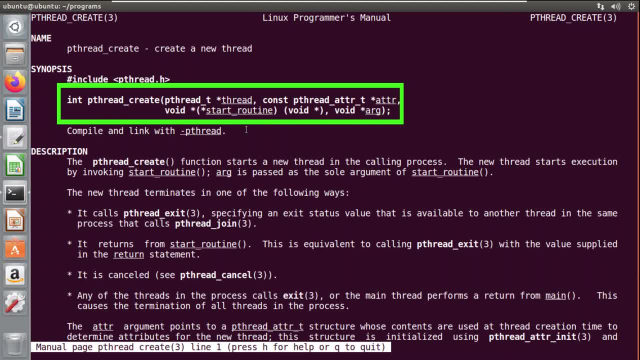 this function takes actual four parameters. the first parameter takes a pointer to pthread underscore t. second parameter is nothing but the attributes that we require while creation of a new thread. but if we want default attributes then you can pass a null here. i have also passed null as my second parameter. the third parameter is nothing but the task that our 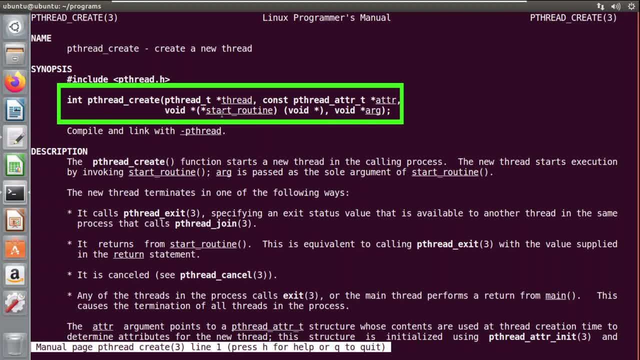 process will be performing. so we have to pass the function name or you, whatever you want to pass the function name or you, whatever you want to pass the function name or you module you have creating. and the last parameter, that is the fourth parameter, is nothing but the. 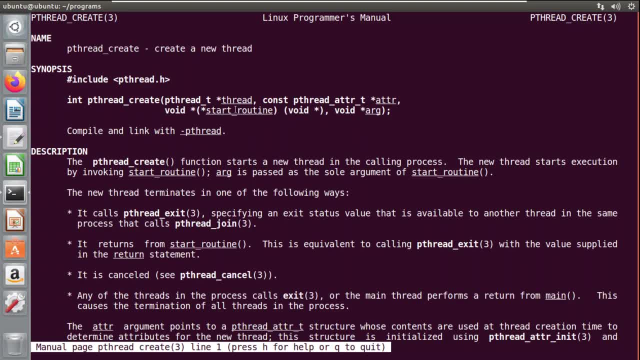 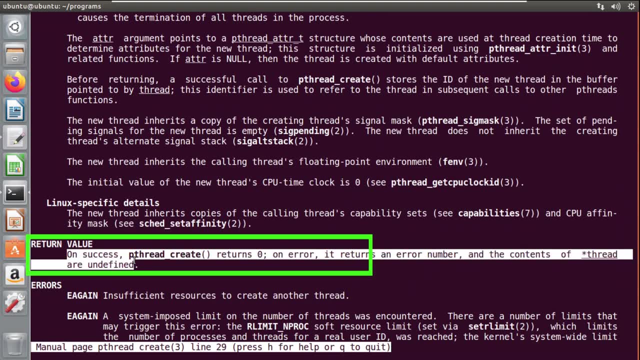 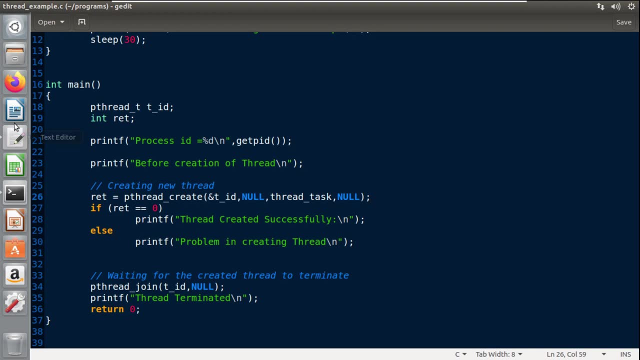 arguments that you want to pass to this function that we are going to create now. if you scroll down here, you will get a message that on success of this function you will get a zero. otherwise you will get an error. so now let's go to my program again, and here i have created a function. 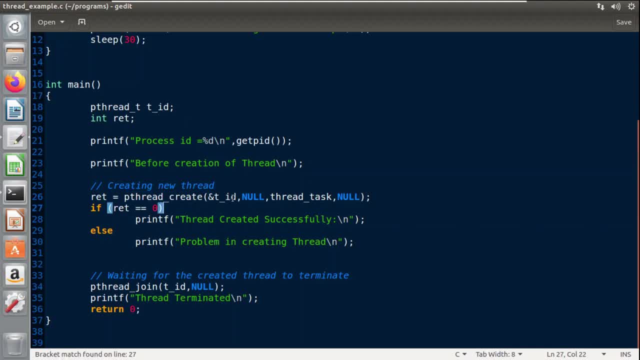 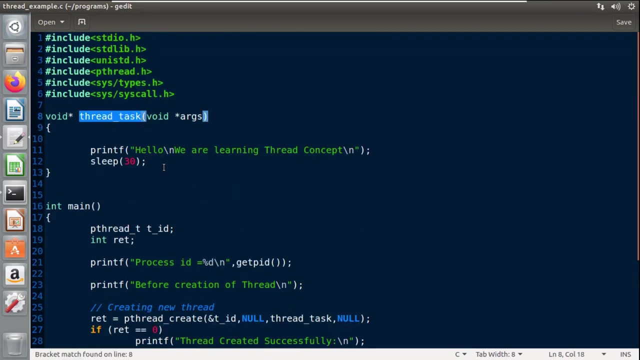 that is a pthread underscore create and first parameter i have passed as a pointer to pthread underscore t. second parameter is nothing but the attributes that i am considering the default attribute. so i have passed a null here. third parameter is nothing but the function that i have created here. so thread task is nothing but the function that i am going to assign to my 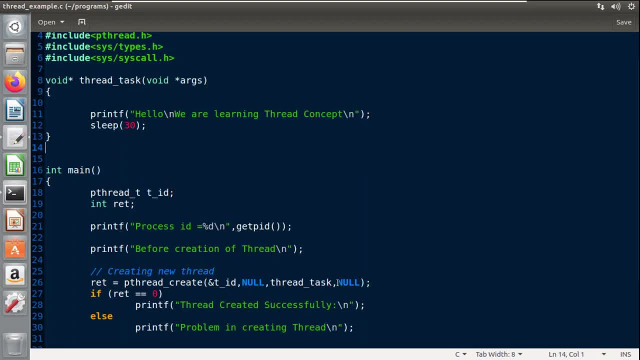 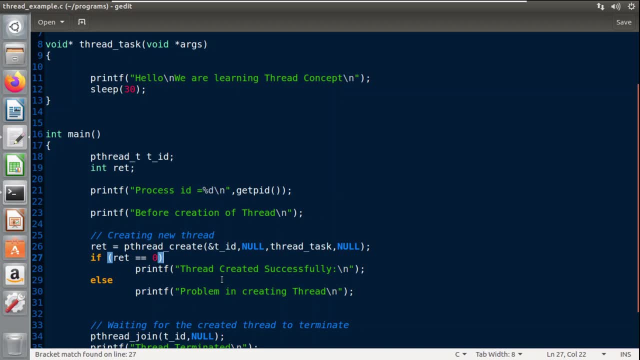 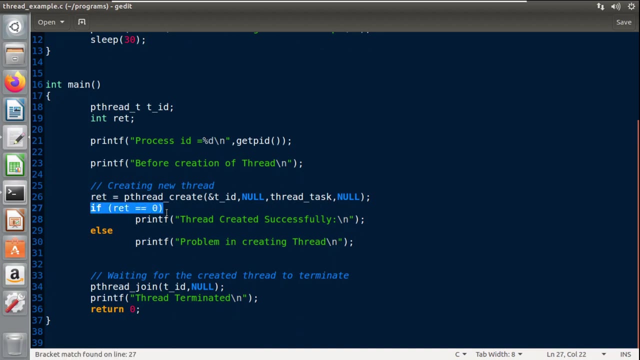 process here and i am not passing any arguments or to my function. so i have passed a null argument here. now i am going to check whether my thread has been created properly or not. so i am considering the return value and i have checked the condition, as if written value is equal to equal to zero, then my thread has been created successfully. 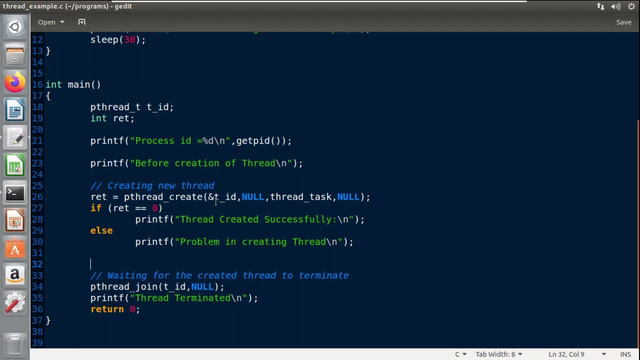 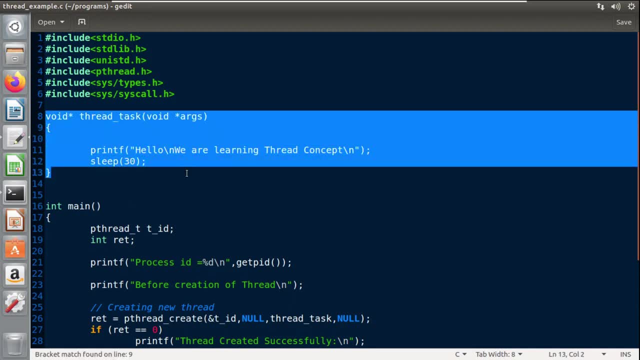 otherwise there is a problem in creating my thread. now let's go to the function that we are going to run. so i have created a simple function wherein i have just passed my message that we are learning the thread concept, and i have called a sleep function here so that we can check the 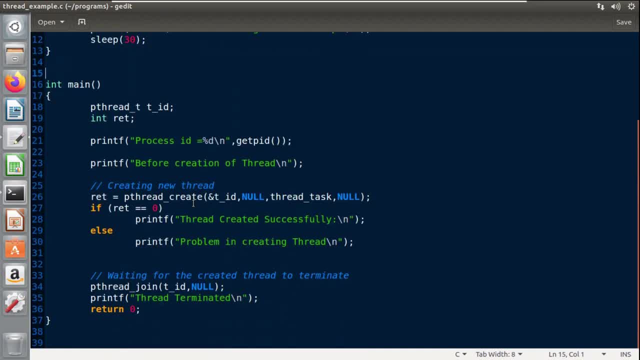 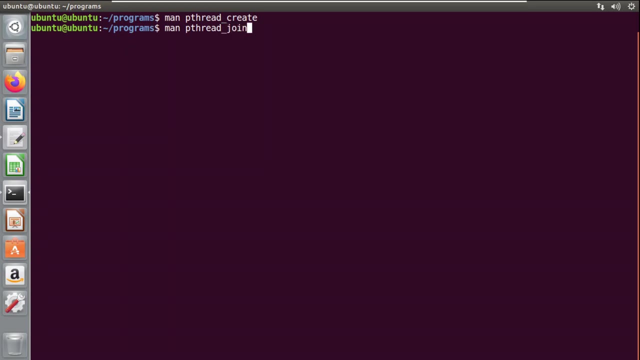 status of my thread while checking the output and now after creating my thread, i have called another function here, that is a pthread join. now we will check the manual page of this pthread join. so pthread and underscore join. so if you check here it is nothing, but we are checking whether my thread 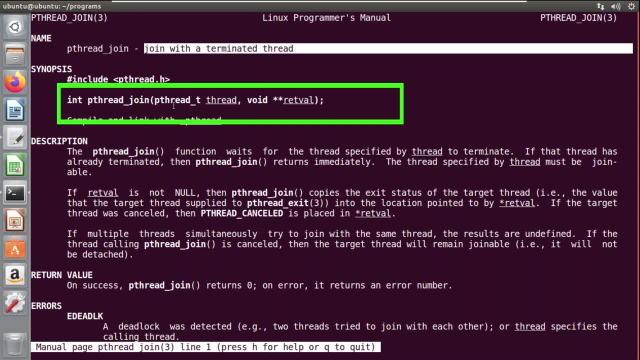 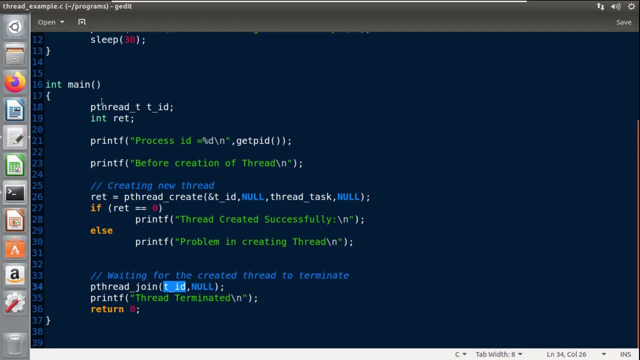 has been terminated or not, and uh to this function i have to pass uh the pointer again of a pthread underscore t and uh, the return value. right now i am not passing any return value, so in my function i have a passed a value of a pthread underscore t. that is a tid that i have called. and the second: 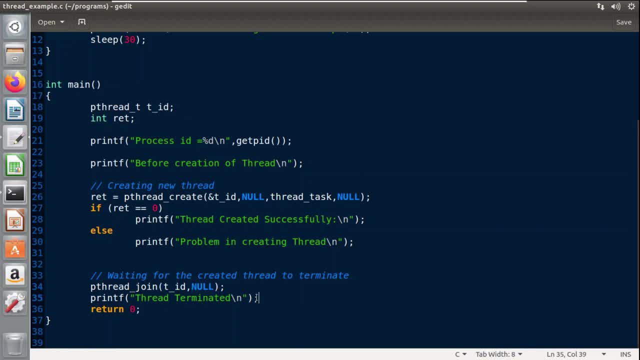 parameter is nothing but a null. so i have not passed any return value here. and lastly, i have printed a message. that is my thread and i am going to check whether my thread has been terminated or not successfully. so basically, this pthread underscore join function is used to wait. 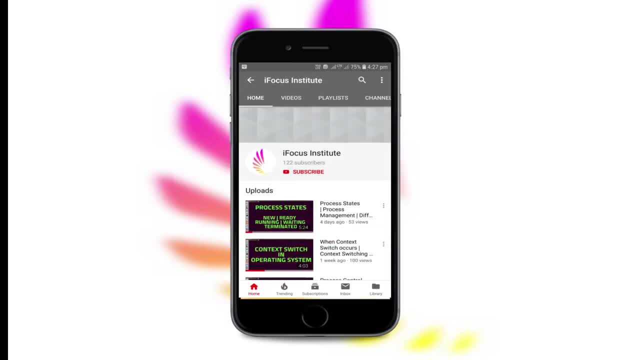 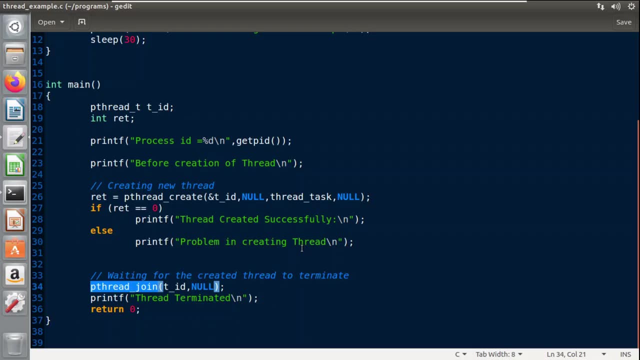 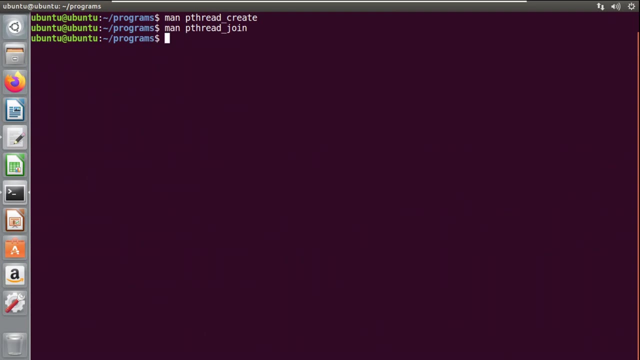 until my created thread gets terminated. to get the information about the tutorials, press the subscribe button and click on the bell icon to get the notification. now we will run this program. uh, so we'll go to your terminal here. i am running the program by using the gcc compiler and my file. 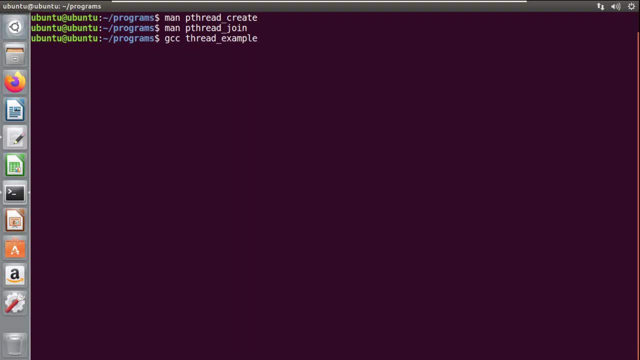 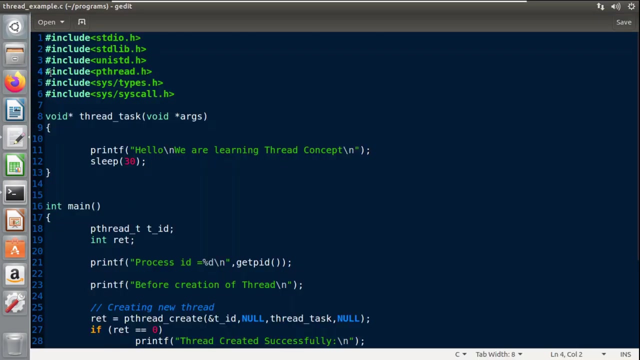 name is a thread underscore- example: dot c. i want the output by the name thread example again, and so now we will check the output. oh, there is an error. if you observe here that i have getting an error as a undefined reference to pthread underscore, create now what is this error? actually, i have used the header file by the name pthread dot h, but while we 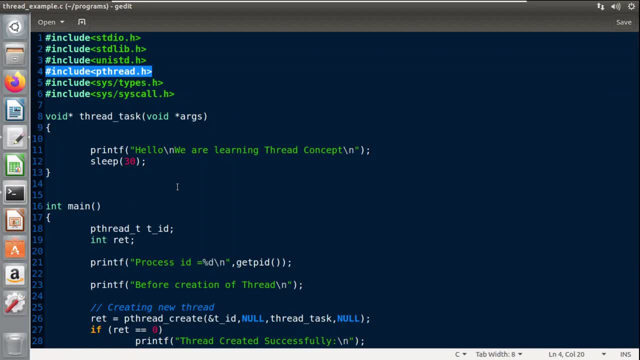 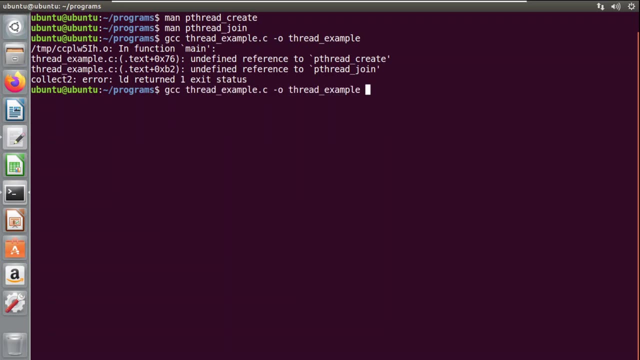 are compiling our program, we need to tell a compiler that we want to execute this program, this entire program, by using the p thread library. so how we have to do it? during the compile time, during the compilation, we have to pass a argument, that is, a hyphen, l and p thread, which means that 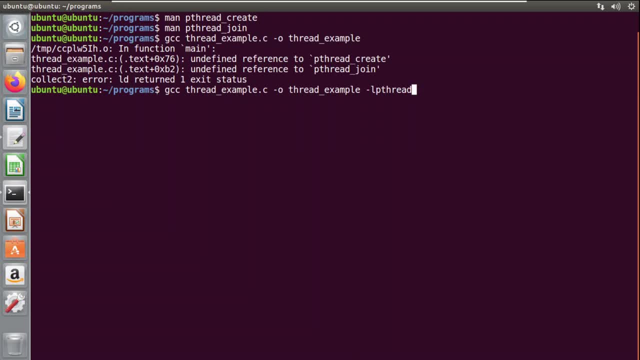 we are telling our compiler to include the pthread library for my program. so now, while running the program, it has been compiled successfully. so here we are, running the program and now i am going to successfully now check the output. so if you observe here the process id that i am getting, 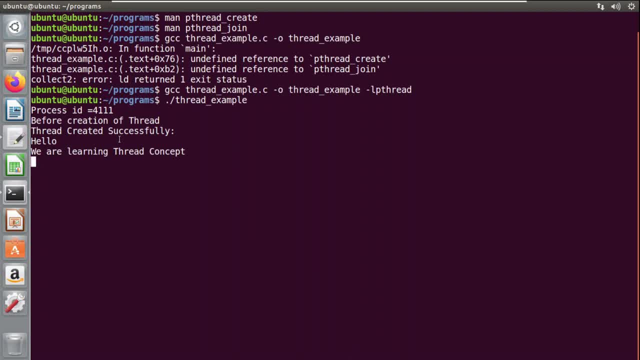 is 4 1, 1 and our thread has been created successfully and we have entered our function or, we can say, the task that we want to perform now. here i am going to open a new terminal again and i am going to check the status of my thread. so how to check the status is ps, hyphen t. 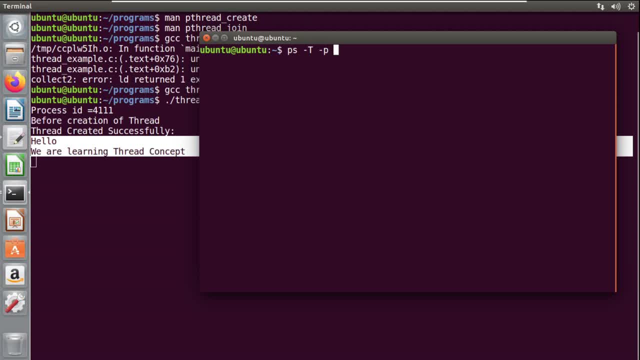 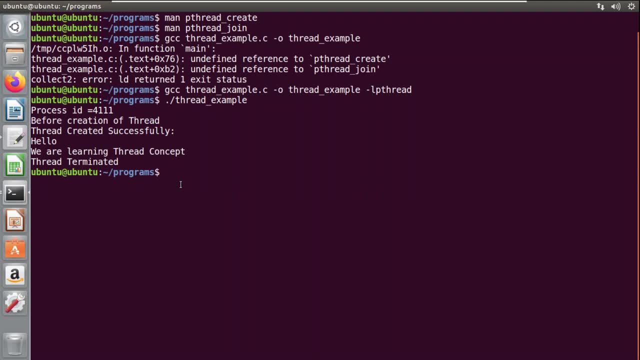 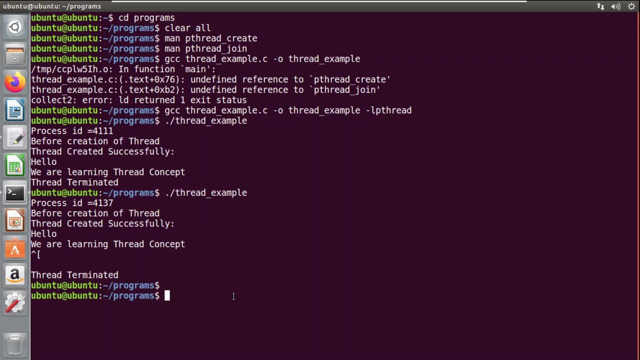 hyphen p, and we have to mention the process id, which is 4 1 1 in my case. oh, my program has been terminated, so i will run my program again and then i will show you the status. by mistake, i press some key and so my thread got terminated. so i will run my program again. and now i will. 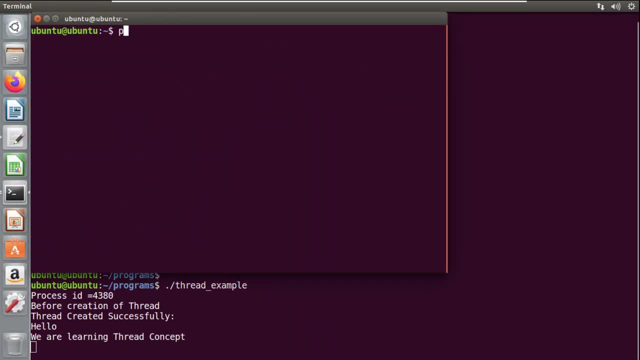 open a new terminal here where i will be running a command to check the thread. so ps hyphen t immersize. and here i am going to open a new terminal again and i am going to press 새 esp Scriptures. so ps hyphen t inappropriately. and here i am going to check the status of my thread. so ps hyphen t. 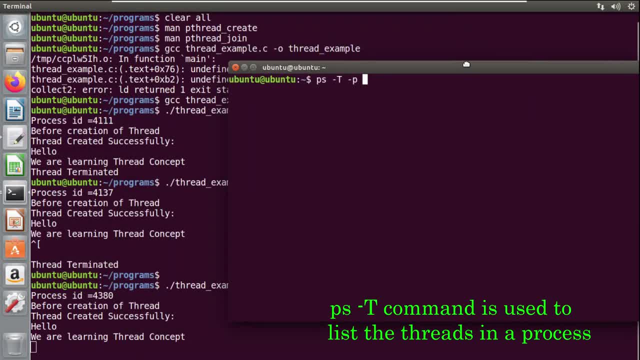 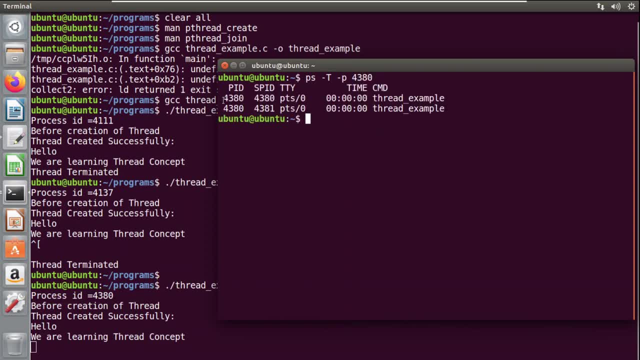 hyphen p and then my process id, which is right now 4380, so 4380. now, if you observe here this 4380 is nothing but my process id, that is the pid, and it has created two thread right now, which is 4380. 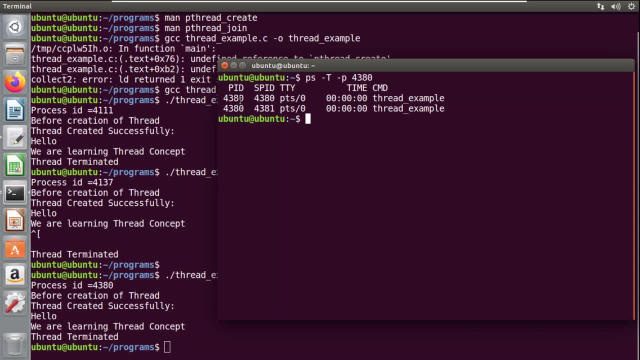 and 4381. if you observe here properly, the process id is same, that is, 4380 remains same. but i have created two threads here. now. this first thread, that is 4380, is nothing but uh, the same as my process id, and this uh, 4381, is nothing but the task or the function that i am performing. 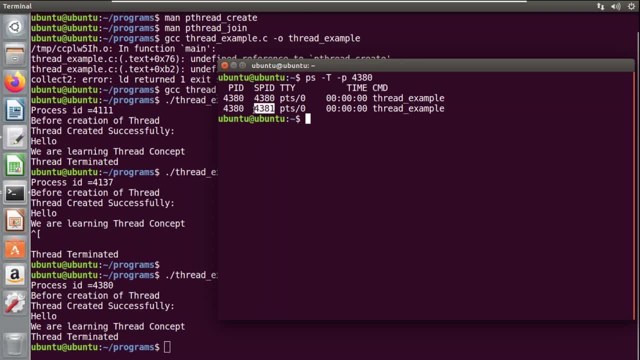 in my program. so actual function that i am going to perform is by using the thread id, that is 4381. now, if you observe in this terminal, my process has been completed and my thread has been terminated. so we will check the status here again. and if you observe here: 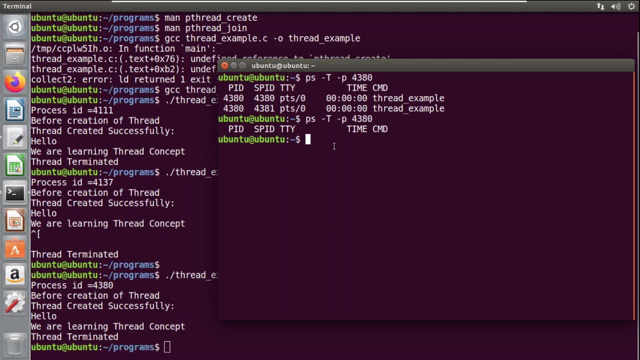 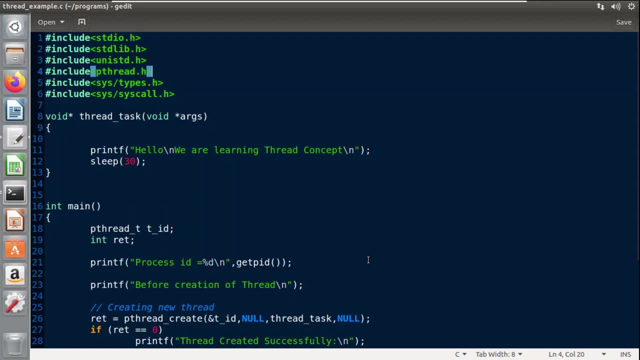 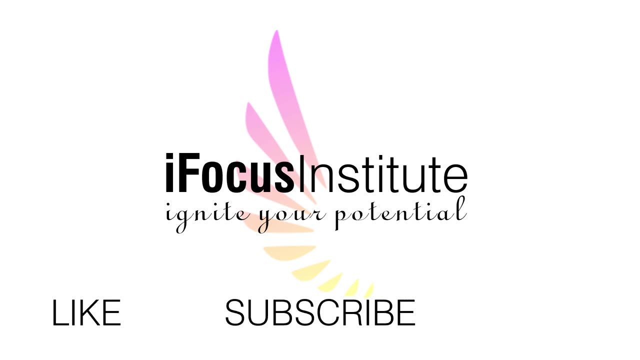 i am not getting any output, so my thread has been terminated properly. so, similarly, we can assign multiple tasks to our process and these, each task- will be considered as a thread.